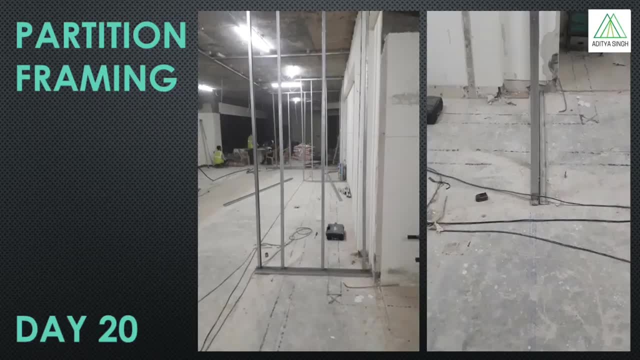 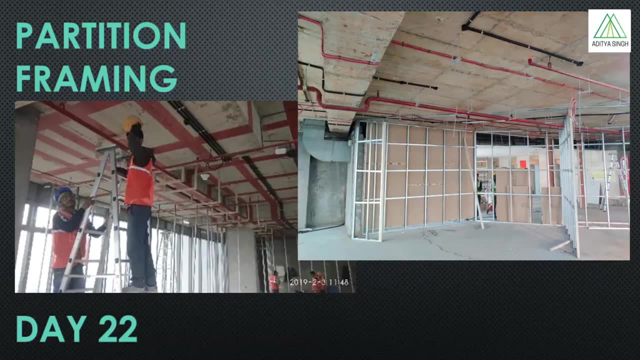 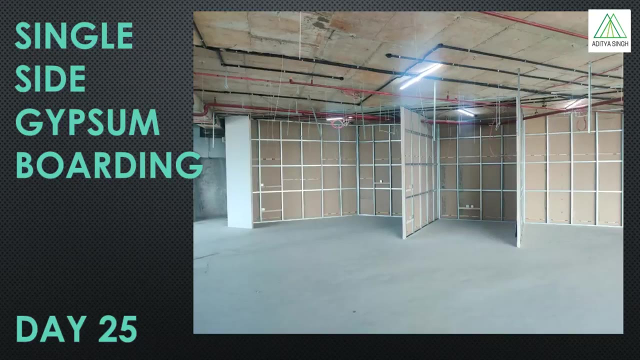 Partition marking is followed by installation of G-studs framework for partition. As a general practice, the center to center distance between the horizontal and vertical framing members is 600 mm. Once the framing is completed, single-side gypsum boarding starts. This involves fixing gypsum board on one side of framing. 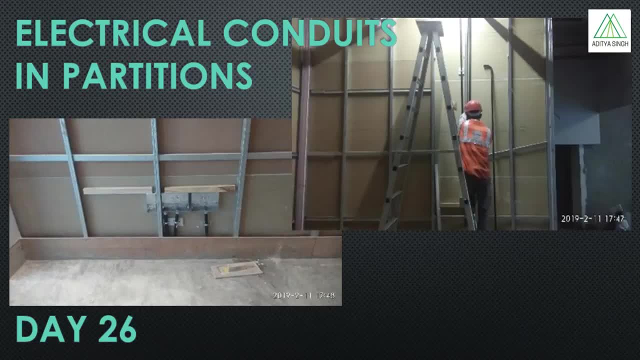 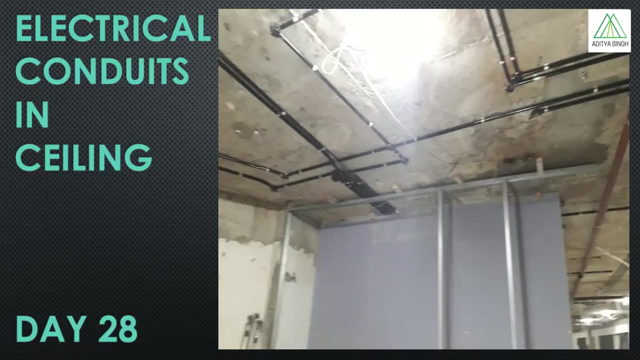 Next, the partition. Internal services like electrical and data are planned and accordingly conduits and raceways are installed in the partitions from the other side. In parallel, the conduits in ceiling for power and data are also installed. Once the conduit installation is completed in partitions, acoustic insulation is filled. 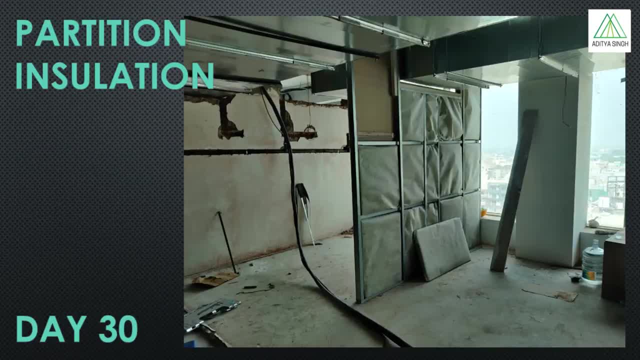 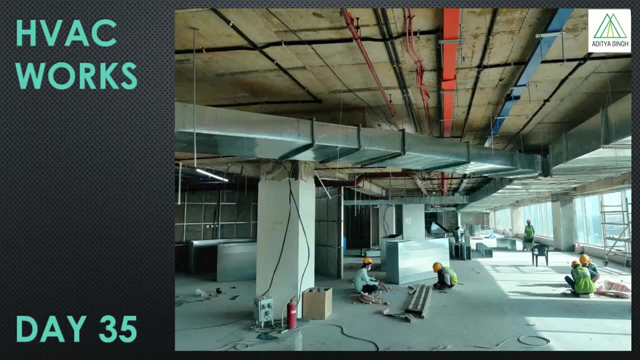 between the framing, so that there are no cavities left. While all the works is happening, the HVAC and firefighting works are also going alongside. The prefabricated ducting is for the design is installed first. Next nitrile rubber insulation is glued on it, which has two benefits, as it does not, 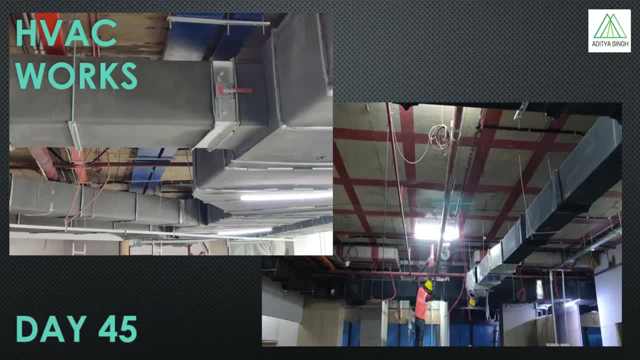 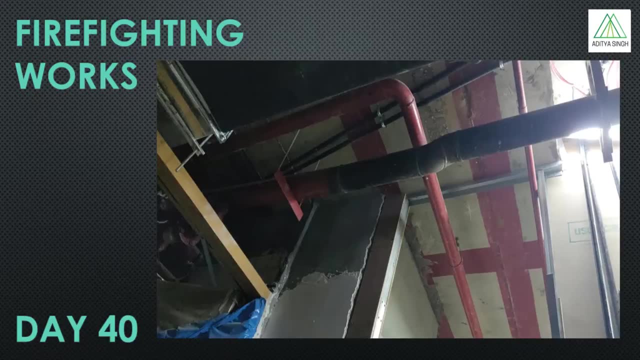 allows the cooling loss and also prevents from sweating on ducts due to condensation. Firefighting works involve running sprinkler pipes all over the ceiling and then installing sprinkler heads and finally testing the system for required pressure performance. This is mandatory requirement for getting the fire safety clearance. 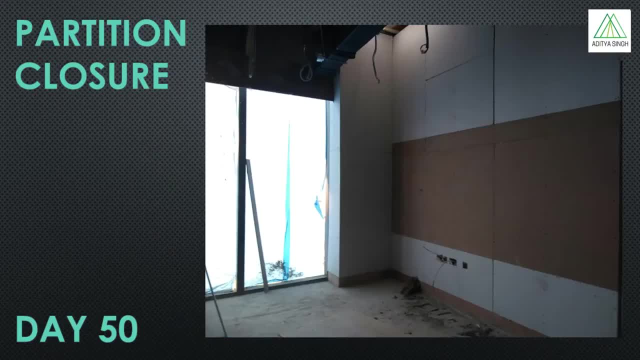 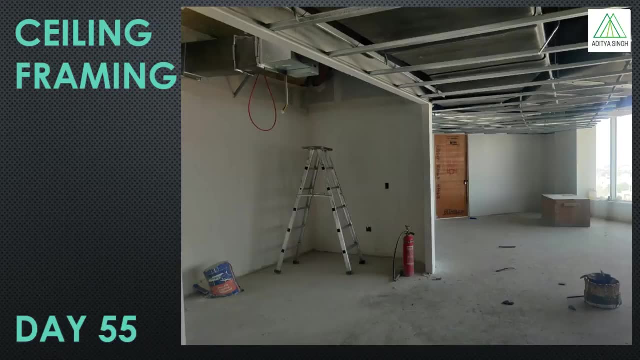 Once the partition insulation work is completed, partitions are closed with gypsum board from other side as well. Ceiling framing work is the next activity. This involves the installation of ghee ceiling framework which is supported from the ceiling supports, from the structural slab and from the sides of partition. 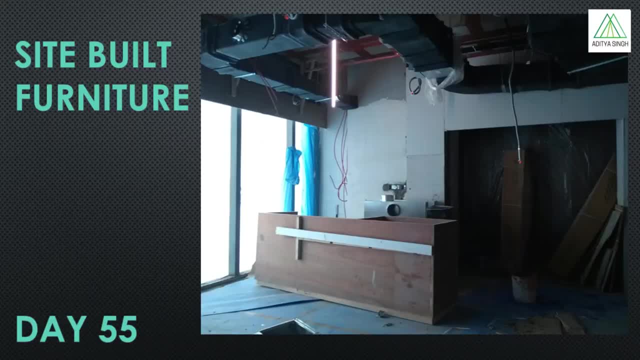 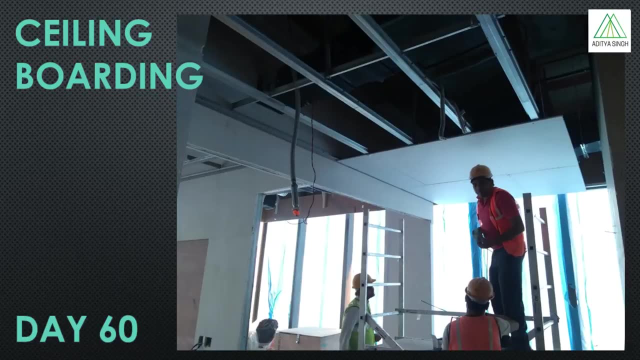 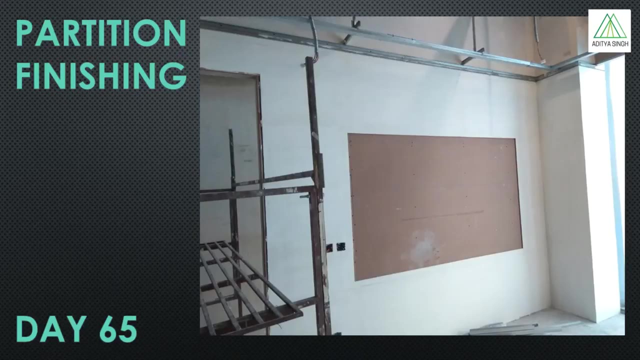 The built-in furniture starts getting build alongside these works at site itself, After completion of ceiling framing works. the ceiling boarding is done by screwing gypsum boards to the frame. The partition and ceiling finishing works are the next activities. These involve jointing and taping of gypsum boards and is finished with a drywall compound. 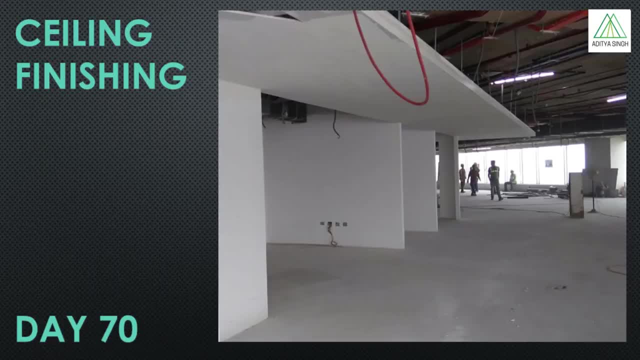 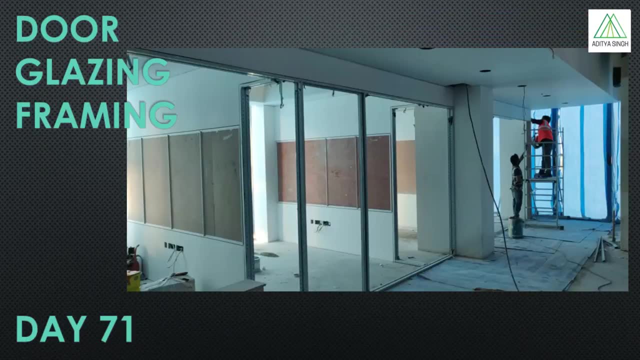 followed by sanding. Once the smooth surface is achieved, primer coat is applied to take on the first layer of paint. The aluminum partition works installation is the next activity. This is basically the installation of framework which will take on the glazing and doors of